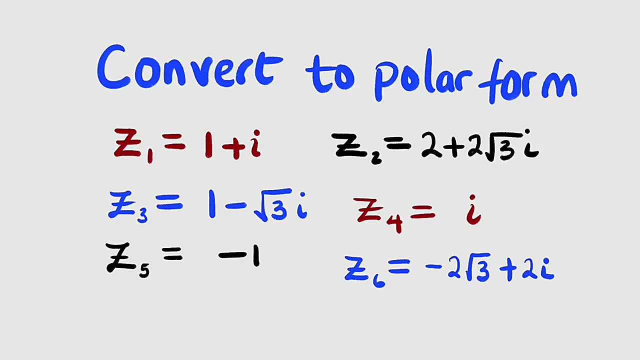 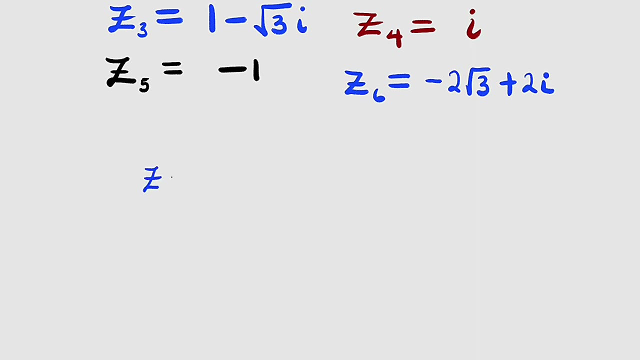 Hello, good day viewers. In this tutorial we are going to learn how to convert a complex number from a rectangular form to a polar form, And we have six problems right here. But before we start let me explain this. Remember the general form, z, equal to a plus bi. In our previous lesson we 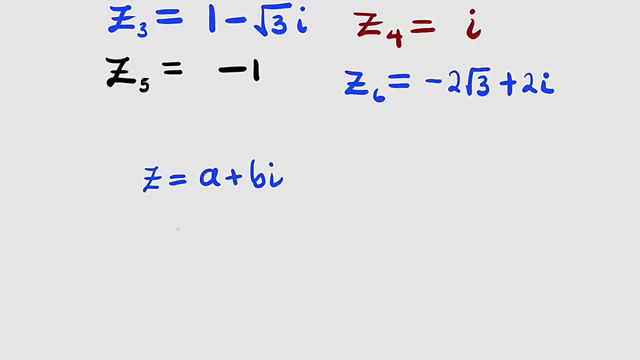 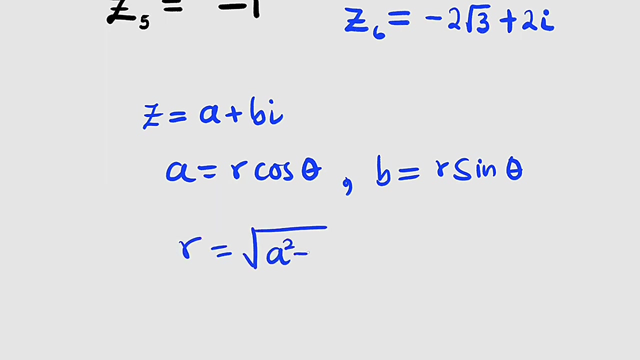 have learned that the real part of a complex number can be written as r cosine of theta Right, While the imaginary part, which is b, is equal to r sine theta, Where r can be of 10 by taking the square root of a squared plus b squared, And theta is just equal to the tan. 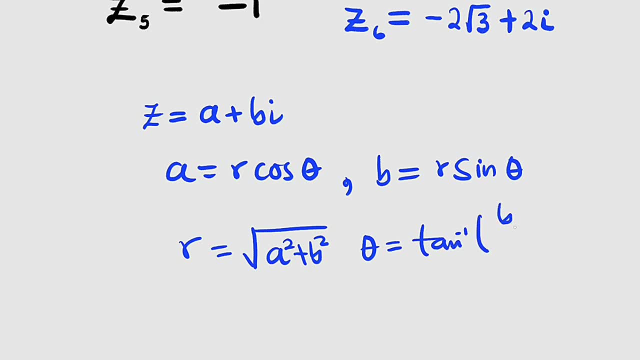 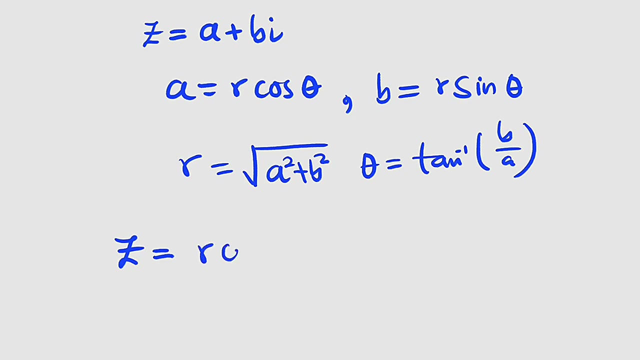 inverse of what b divided by a. So if this is the case, how can we transform this complex number to a polar form? By just substituting a and b. So z will be equal to a, which is r cosine theta. then, plus i multiplied by b, which is r sine theta, You can see we have r. 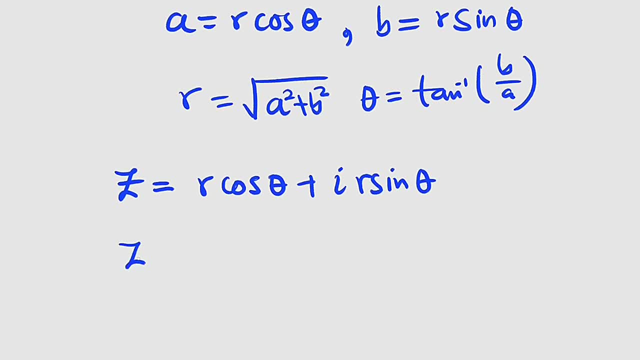 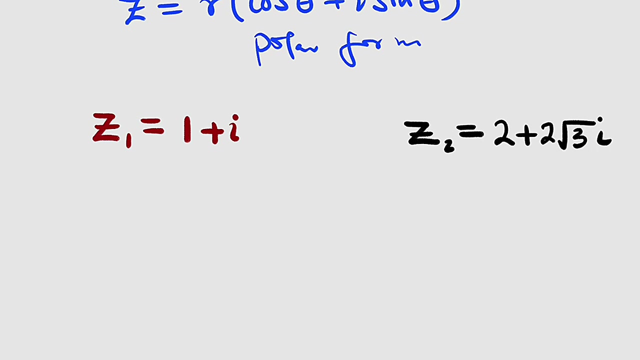 common. so we can factor it out. So z, finally, will be equal to r multiplied by cosine theta, then plus i sine theta, And this is just the polar form. So now let us apply this idea to transform the following complex numbers into polar form. All right, here are our first two. 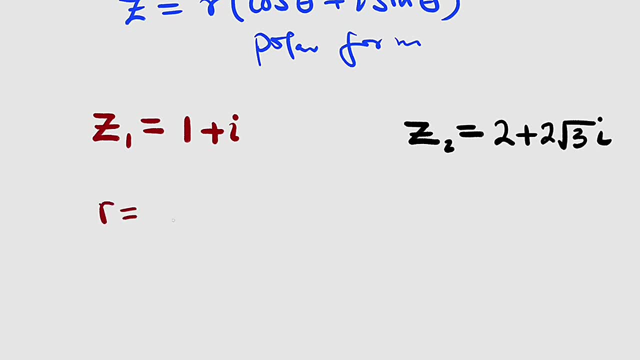 problems. Let's start with r. r will be equal to the square root of a squared plus b squared, And we have a as 1.. We have b, which is the coefficient of i, as also 1.. So 1 squared is 1.. 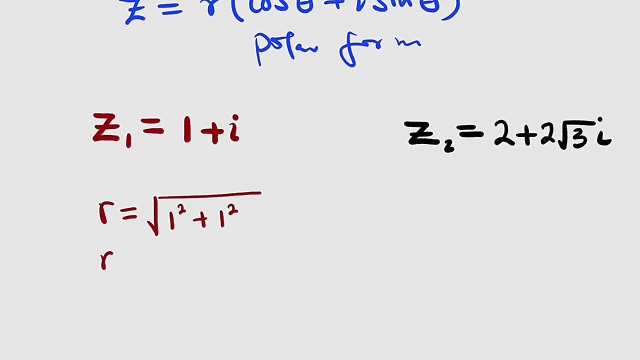 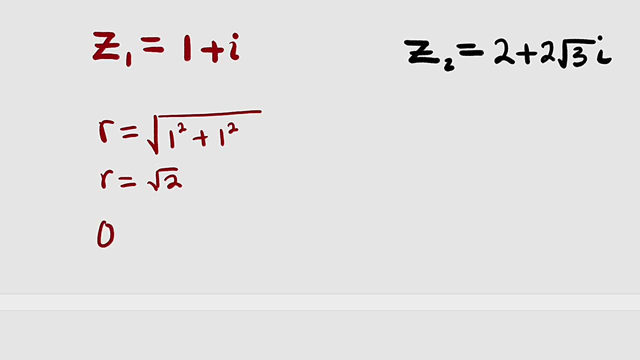 1 squared is 1.. 1 plus 1 is 2.. So finally, r will be equal to just root 2.. So what about our theta? Theta is equal to tan inverse of b, which is the coefficient of i 1 divided by the. 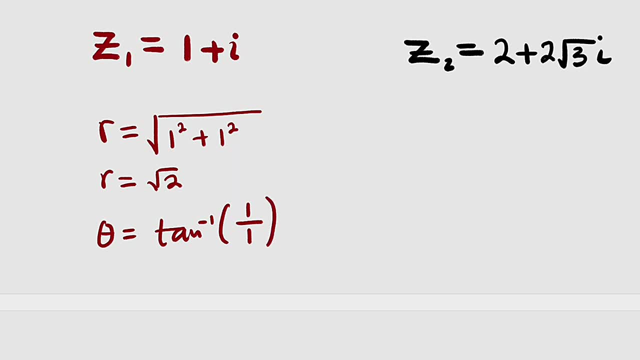 real part, which is also 1.. 1 divided by 1 is 1.. And tan inverse of 1 is pi by 4 or 4 to 5 degrees. So let me use radian here. So theta is equal to pi by 4.. Therefore, 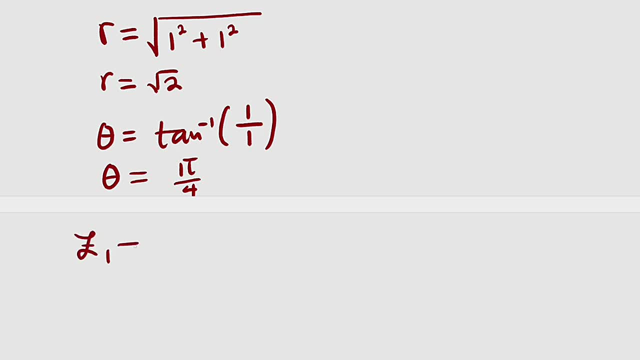 our complex number will be z1 equal to r, which is root 2. Then multiply by the cosine of that angle, which is pi by 4.. Then plus i, multiplied by sine of that angle, which is also pi by 4.. Now the second one: We have z equal to 2 plus 2. 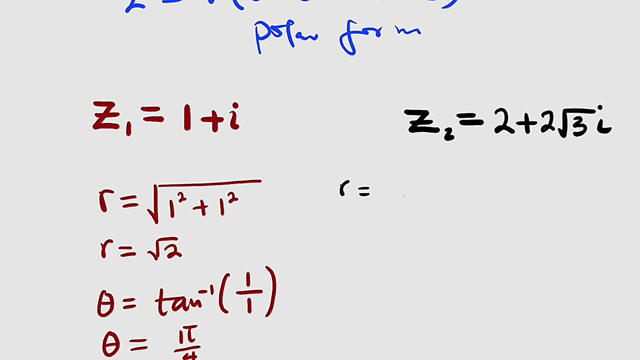 root 3i. So the radius will be equal to the square root of a squared, which is 2 squared, plus the imaginary part, which is 2 root 3. all squared, 2 squared here is 4, and if you square this, you 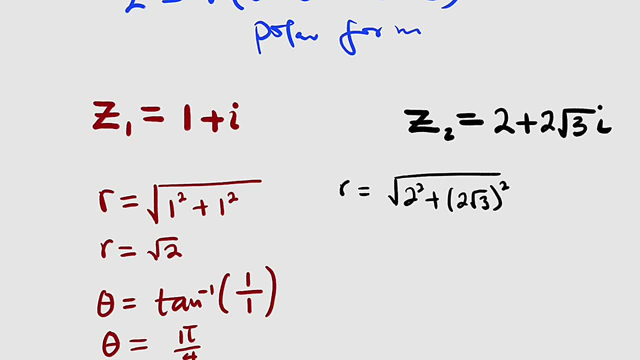 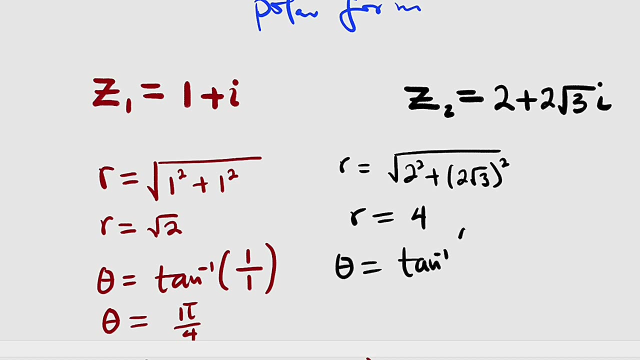 have 4 times 3, 12 plus 4, 16, and square root of 16 is 4.. So we are taking only the positive number, 4.. While theta is equal to tan, inverse of 2 root 3 divided by by 2.. And 2 root 3 divided by 2, 2 will cancel. 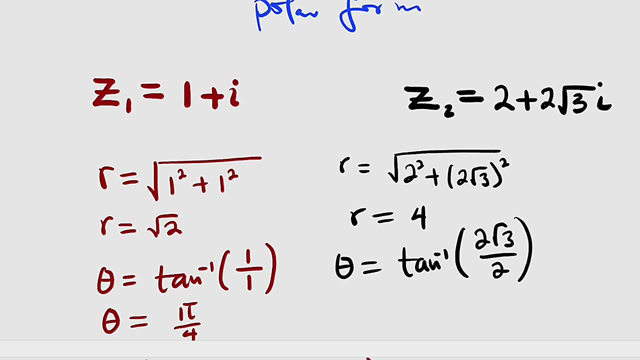 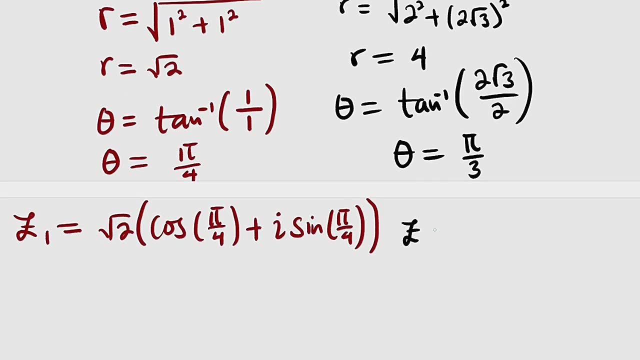 2, leaving only root 3, and tan inverse of root 3 is pi by 3 or 60 degrees. So theta here is equal to pi by 3.. So now let us substitute into the polar form formula. Therefore z is equal to r, which is: 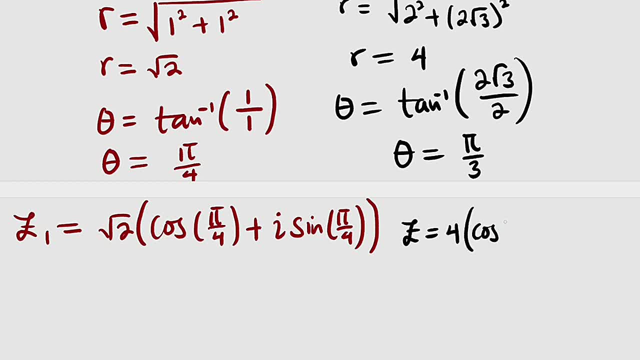 4 multiplied by cosine of what pi by 3.. Then plus i, multiplied by sine of pi by 3.. And this is just the polar form of that complex number. Now let us take the next two. Alright, here are the next two problems. Let's start with r, as usual. 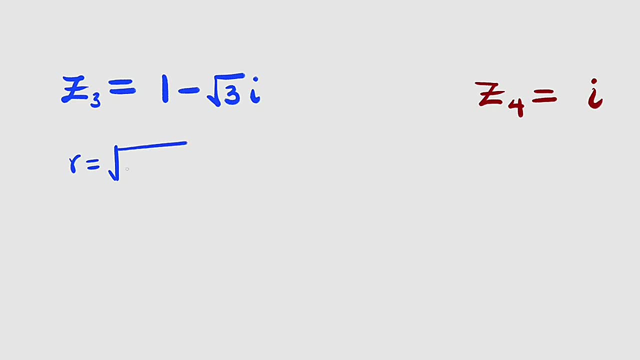 r equal to the square root of real part squared, That is, 1 squared plus the imaginary part. negative root: 3 also squared, 1 squared is 1.. Negative root: 3 squared is 3.. 3 plus 1 is 4.. Square root of 4 is 2.. 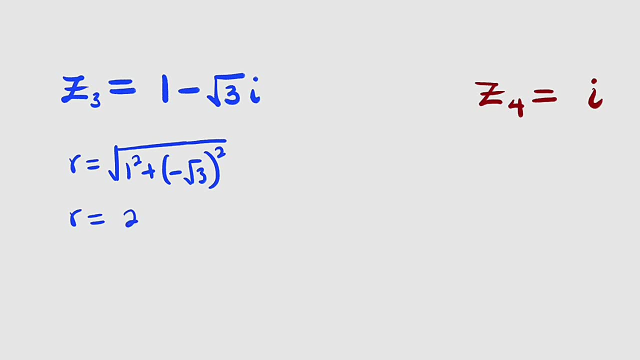 So r is equal to 2.. Remember, we are looking for the distance. And what about the theta? Theta will be equal to tan inverse of negative root, 3 divided by 1, which is the same thing as negative root 3.. And tan inverse: 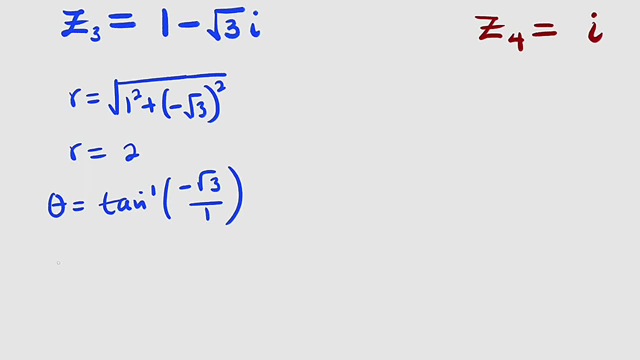 of negative root 3 is the same thing as negative pi by 3.. So theta is equal to negative pi by 3.. But if you wish to take the shortest positive angle, you can add 2 pi, which is 360 degrees. You know, adding a complete circle will not change anything. So if you add 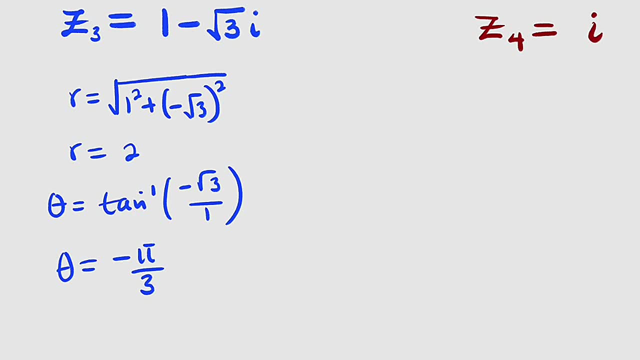 2 pi. to this you are going to obtain 5 pi by 3.. So o 5 pi by 3 is all the same thing. So finally we can plug it into our formula: z equal to r, Our r is 2.. 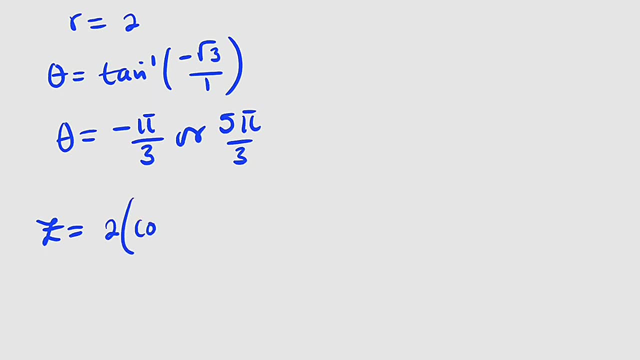 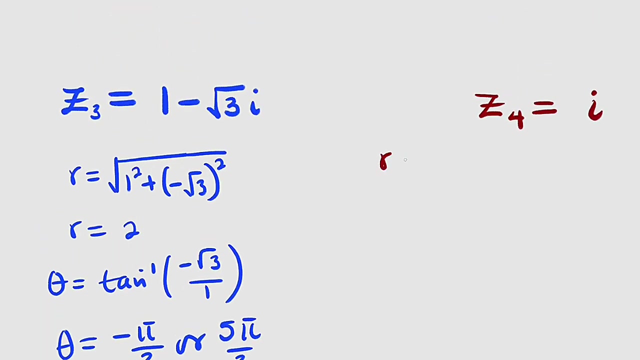 Then multiplied by cosine of 5 pi by 3.. Then, plus i, multiplied by sine of 5 pi by 3.. And hence this is just the polar form of this complex number. The other one we have r to be equal to what Square root of the real part which is absent? 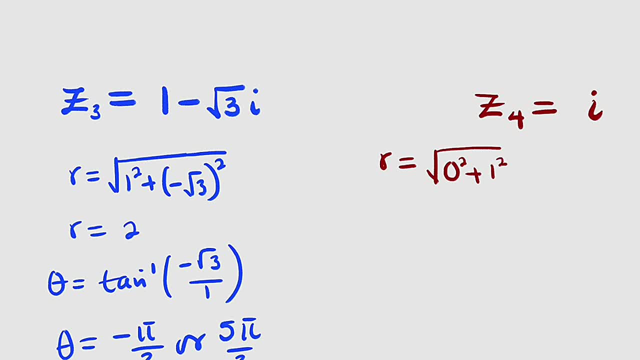 plus the imaginary part, which is just 1 squared 1 squared is 1.. 0 squared is 0.. 0 plus 1 is 1.. Square root of 1 is 1.. Therefore, r is equal to 1 this time around. So what is the angle? 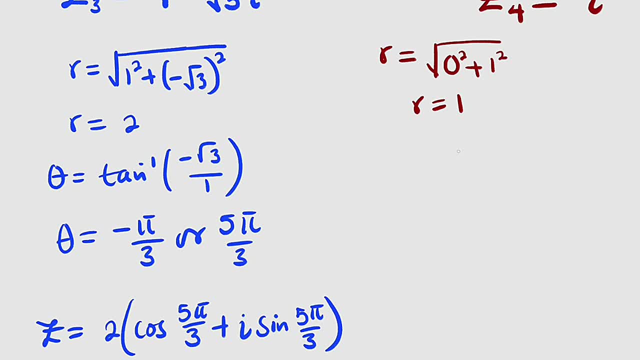 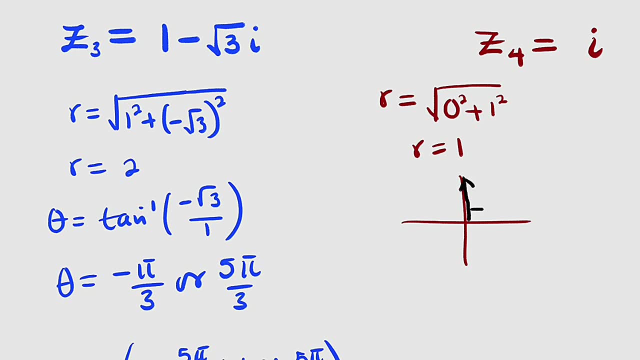 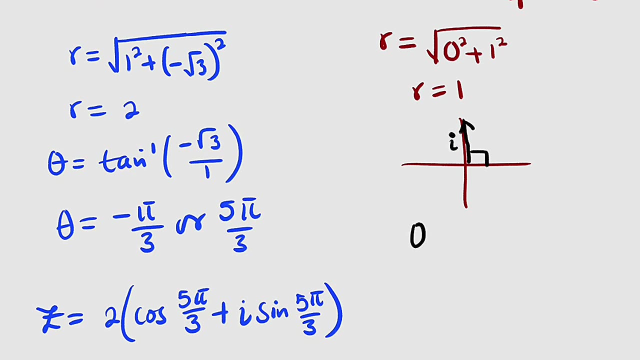 We don't have to compute for anything because, remember, if you have this Cartesian plane, i is just on this y-axis which is completely 90 degrees, or pi by 2, right? Therefore, the angle there is just what: Pi by 2 or 90 degrees. 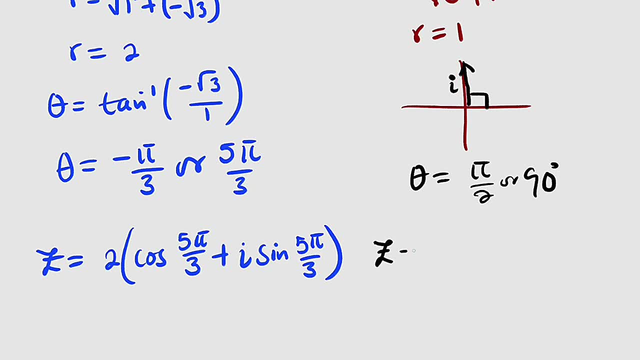 So this complex number to the fuller form is just z equal to r, which is 1.. Do we even need to write it? No, But let me just write it: Cosine of what Pi by 2.. Then, plus i, sine of what Pi by 2.. 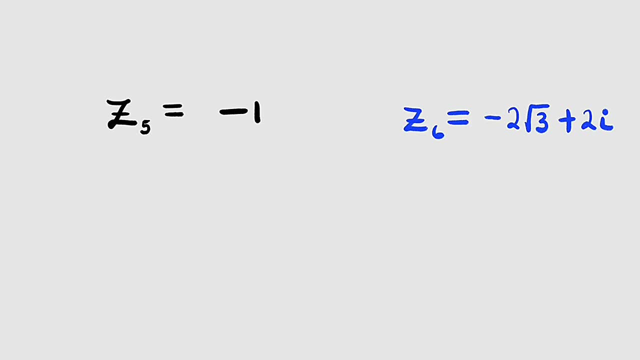 Then the last two. we have z equal to negative 1.. So what will be r, The modulus equal to the square root of the real part, which is negative. 1 squared then plus the imaginary part, which is 0, is also equal to 1, right, So our r is equal to 1.. 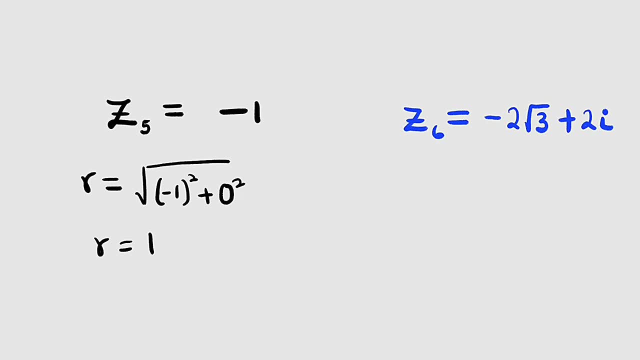 And what about the angle? The angle is 100.. So the angle is 180 degrees or pi. Why? Because on a Cartesian plane, talking about negative 1, it is on this axis negative 1.. So from the terminal point down to this axis is 180 degrees or pi. 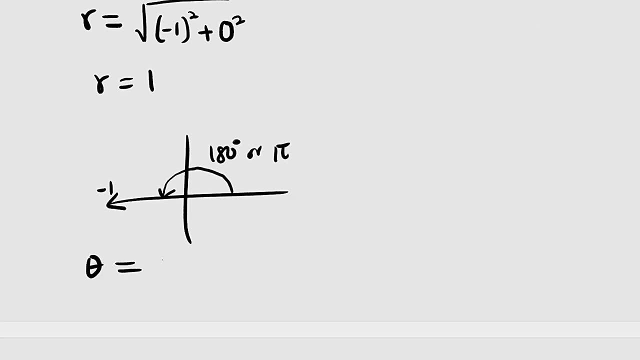 So the angle there of this theta is just equal to pi. So let's substitute everything. Therefore our complex number is equal to 1, which I don't have to write. So the angle is 180 degrees, or pi multiplied by cosine of pi plus i multiplied by sine of pi. 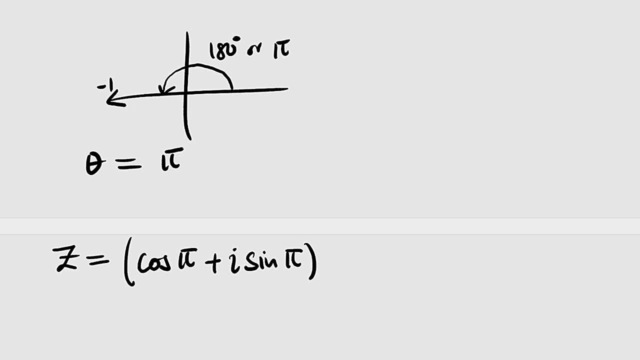 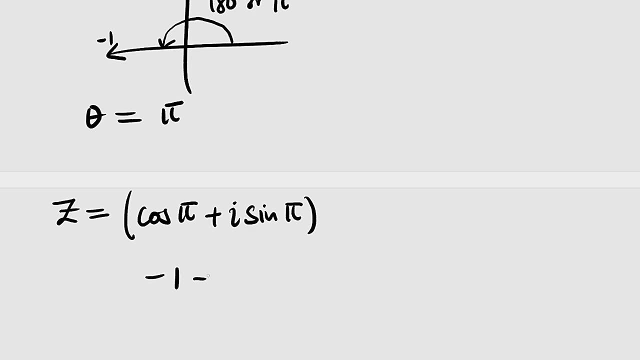 And this is just the polar form of that complex number negative 1.. And if you want to confirm this, let me do it for this. one Cosine of pi is negative 1, remember, plus sine of pi is 0.. So we have, i times 0, which is the same thing as 0. 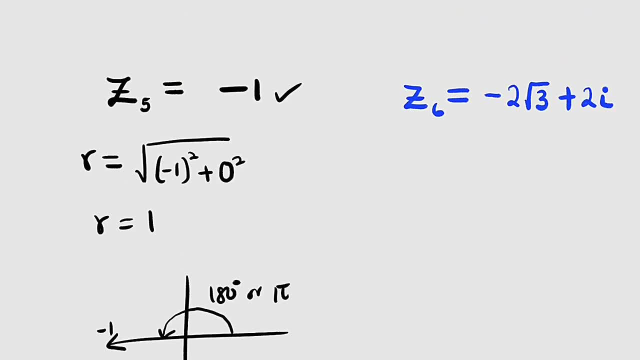 So we have only negative 1. which is the same thing as this one. So let's take the last one. First of all, let us find r equal to the square root of real part. negative 2 root 3 all squared, then plus 2 squared. 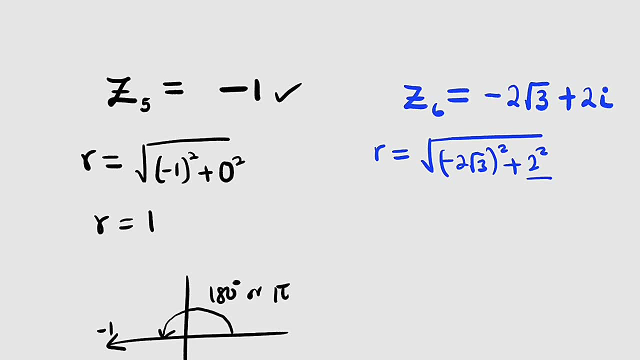 Negative 2 root 3, all squared is 12.. This is 4 making 16.. Square root of 16 is equal to 4.. So the angle theta is equal to tan inverse of what 2 divided by negative 2 root 3.. 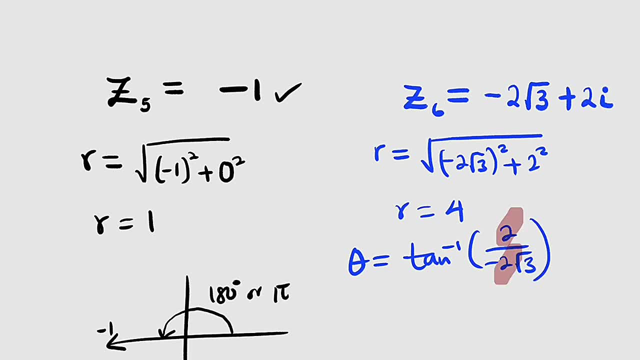 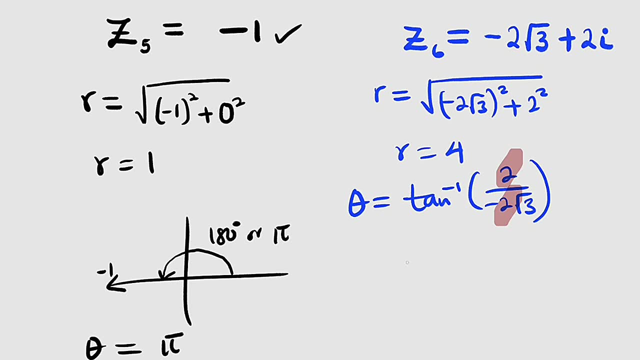 These two will cancel these two. What do we have left? We have negative 1 divided by root 3.. If you rationalize the denominator by multiplying the top and the bottom by root 3, you have tan inverse of what Negative root 3 divided by 3..